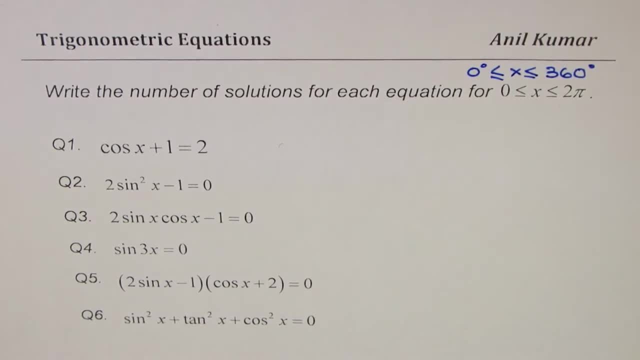 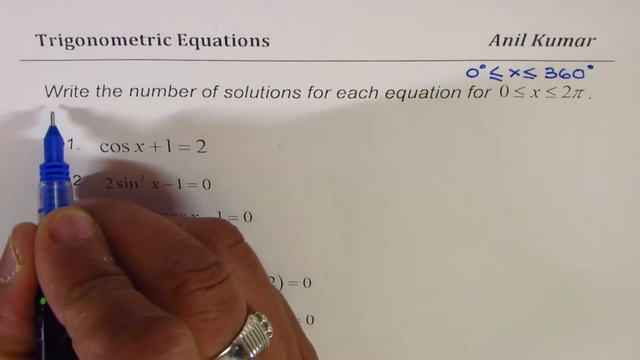 So you will see many questions where we need to write down number of solutions. As you know, trigonometric functions are periodic, So if you are not given any restriction or the domain of your solution, in that case the solutions could be infinite, right? So generally? so we say generally. 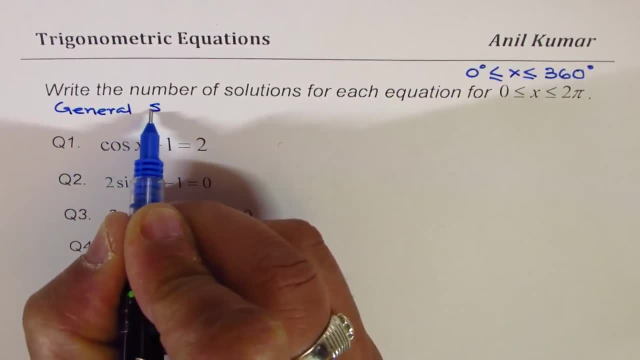 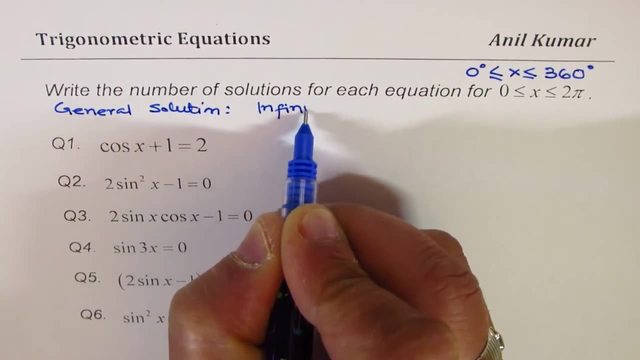 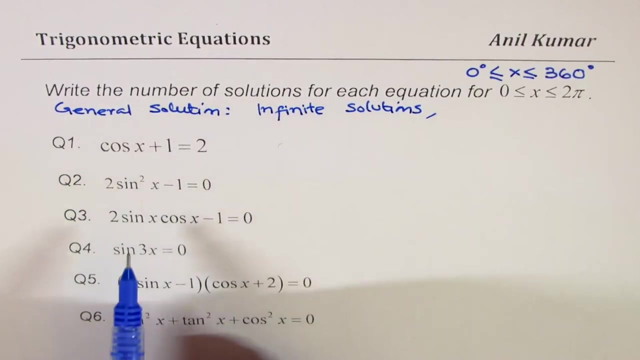 So if I say general solution right, then we are looking for infinite solution Many times right. Why? Because most of these trigonometric functions are periodic correct. Now, in this particular video, we have restricted ourselves to a particular domain. 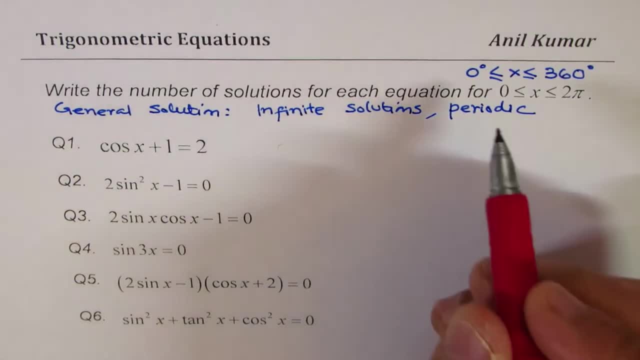 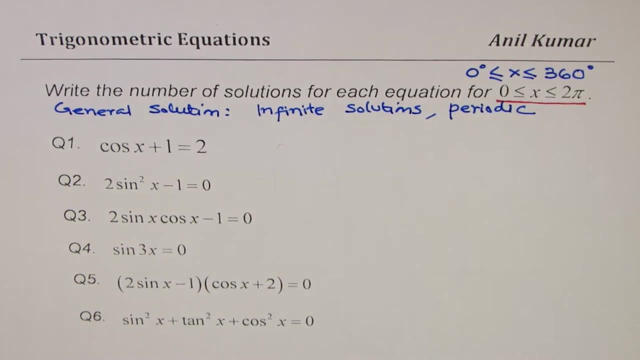 and we are looking for all possible solutions within 0 to 2 pi or 0 to 360 degrees, right, So we will take this one by one. Cos x plus 1 equals to 2.. 2 sin square x minus 1 equals to 0.. 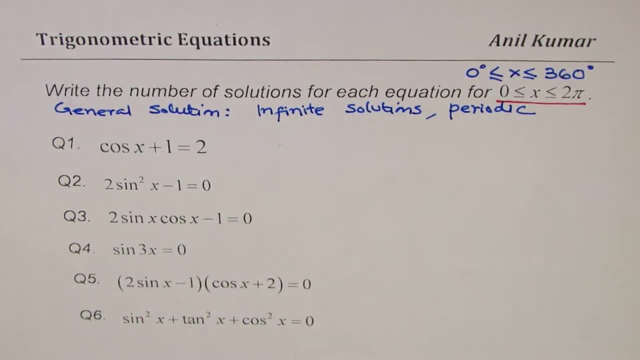 2 sin x. cos x minus 1 equals to 0.. Sin 3 x equals to 0.. 2 sin x minus 1 times cos x plus 2 equals to 0.. And sin square x plus tan square x plus cos square x equals to 0.. 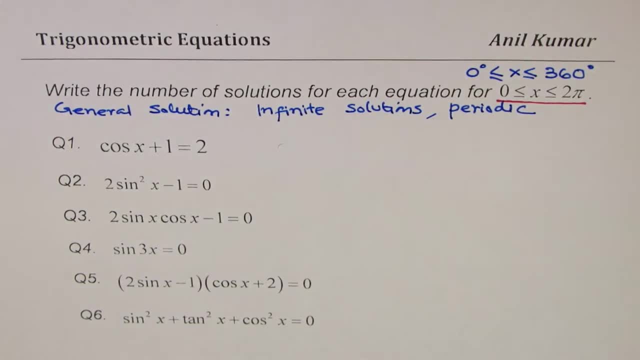 So these are different questions. You can actually pause the video answer and then look at the next questions, So we will take this one by one. So we are looking for infinite solutions into my suggestions. so let's begin with the very first one, which is: cos x plus 1 equals to 2, so 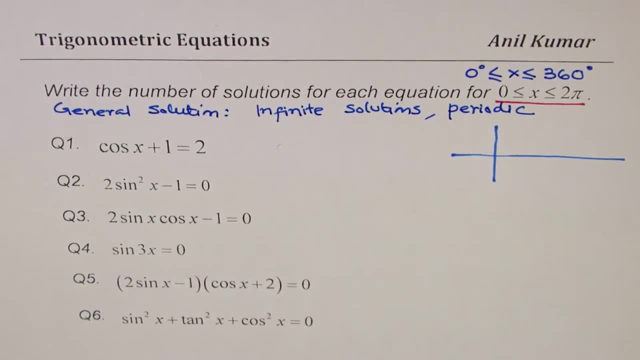 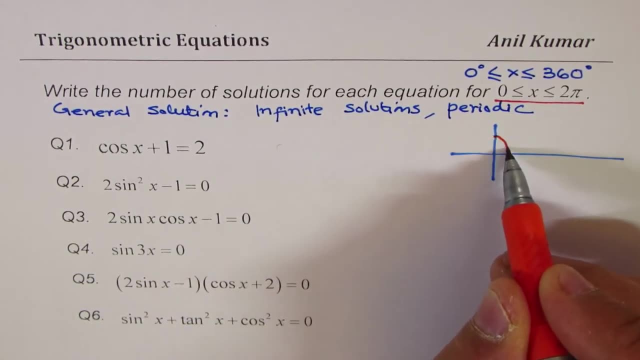 whenever you have to find number of solutions, it's a good idea to sketch the curve. at least have it in your mind, right? so when we say cos x, we're looking for something like this. right? so this is one way. right? so just let me make more. okay, it should be symmetric. this is the axis, anyway. 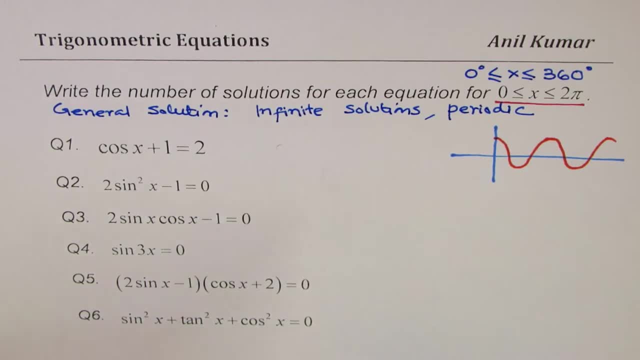 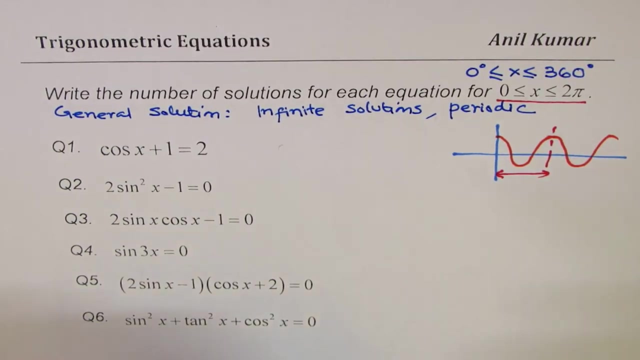 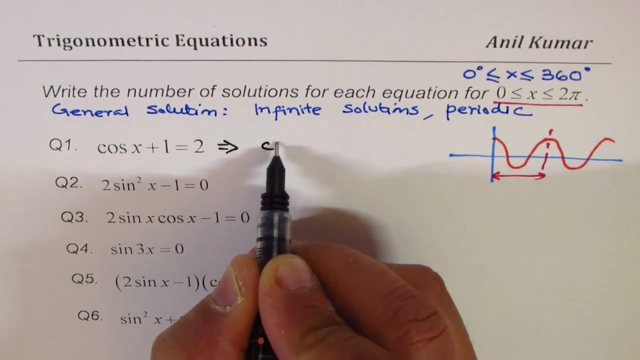 so when we say 0 to 2 pi, we are looking for solutions within this domain. okay, cos x equals to 1 really means I could rewrite this as cos x equals to. I mean cos x plus 1 equals to 2 really means I could write this as: cos x equals to 2 minus 1. right, so 2 minus 1. 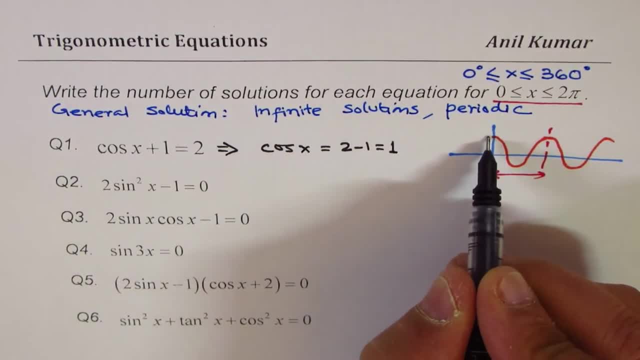 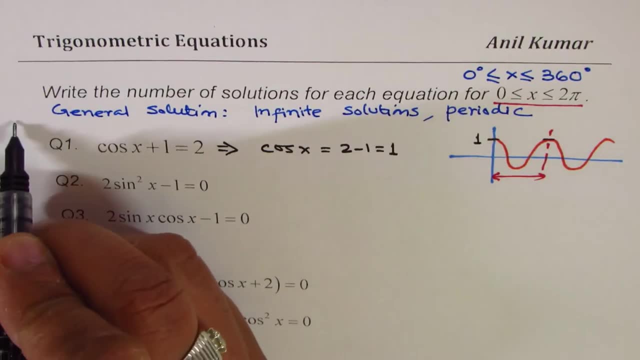 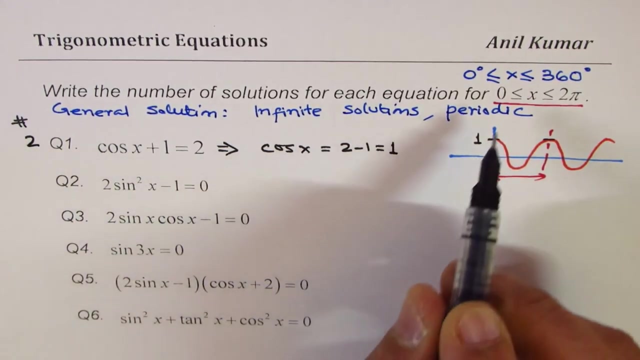 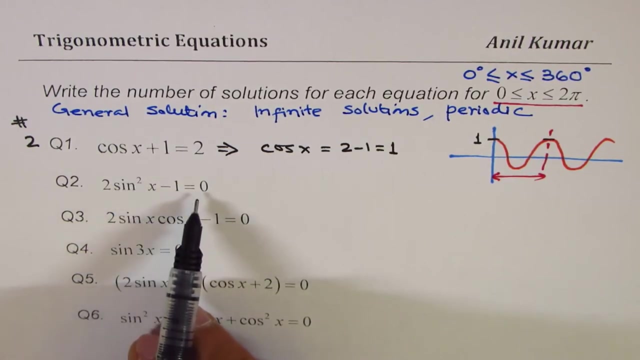 which is 1. now cos x has maximum value of 1. this is 1. so you can see we have two solutions here. so the number of solutions- let me write here number of solutions for each- is 2. so one is at 0, the other one is at 2 pi. the next question here is: 2 sine square x minus 1 equals to 0. so if you 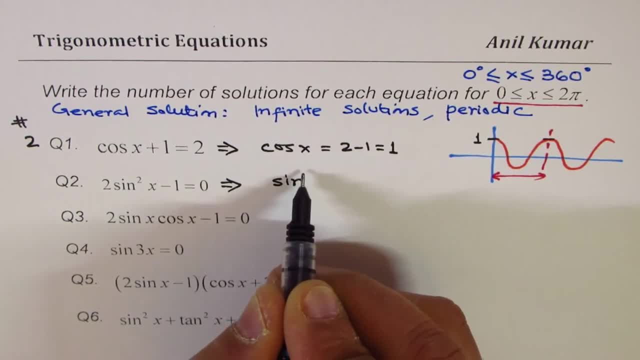 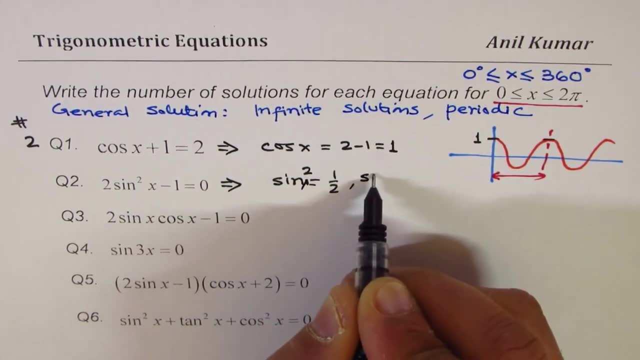 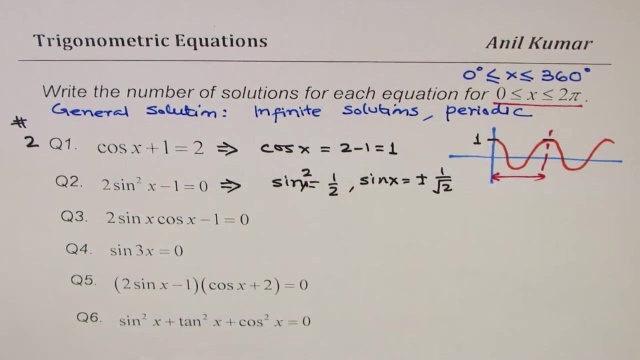 get sine x. let me write in two steps. we have sine square x equals to half, or we have, I mean, sine x equals to plus minus. whenever you do square root, you're looking for 2 right plus minus 1 over square root. now sine x function can be sketched like what it starts with 0 right. 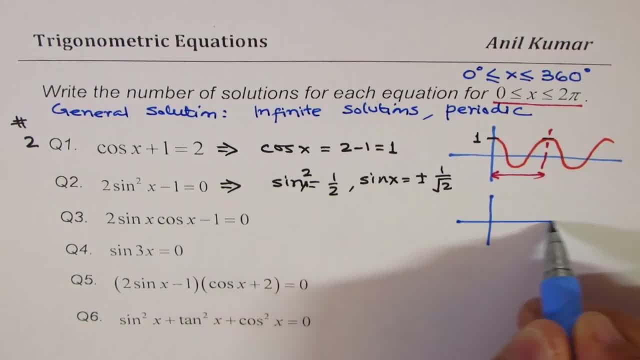 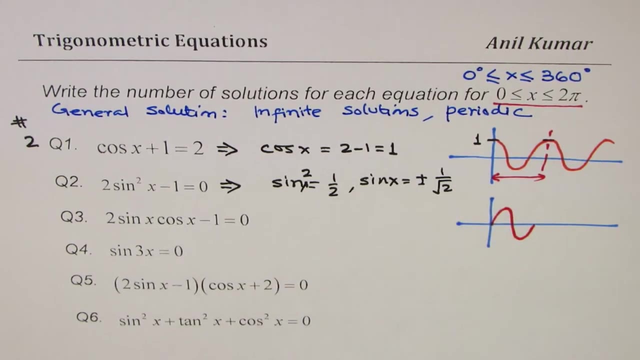 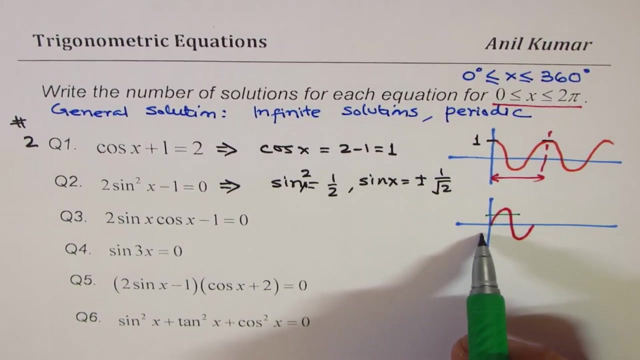 so let me sketch a sine x function here. it starts with 0 and it is kind of like this. so this is one wave. we are looking for some value which is positive as well as negative and is within plus minus 1. so clearly we could have four solutions. you can see this: four solutions. so 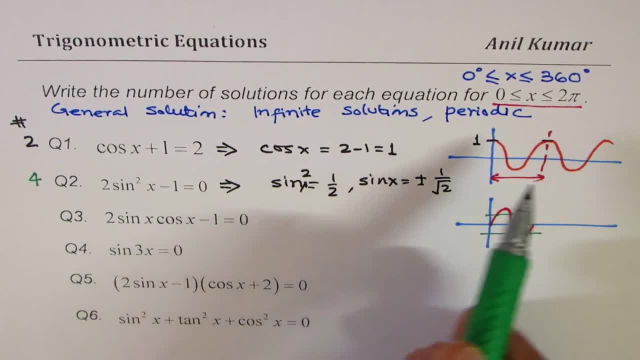 so we have number of solutions as for so. making a wave like this really helps you to understand. how many solutions can you get correct. the next is: 2 sine x, cos x minus 1 equals to 0. now, some of you who have done compound angles, 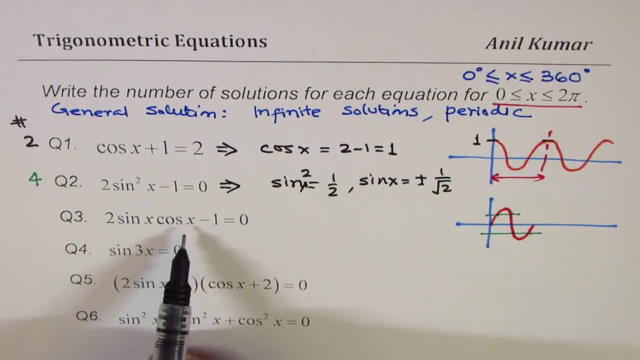 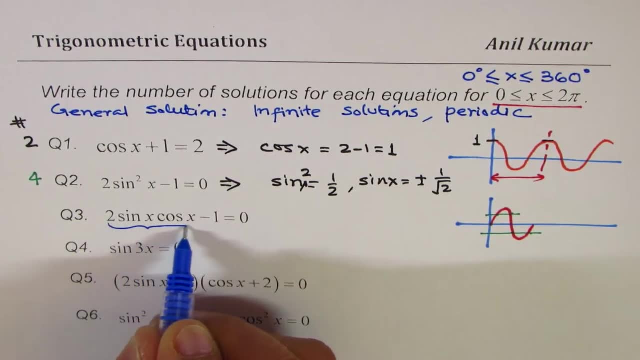 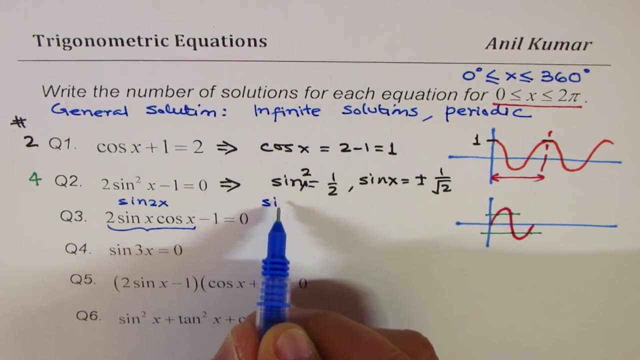 they will know that 2 sine x cos x is sine 2x. right, so we could write this equation as a. this portion here is sine 2x. in that case it becomes sine 2x equals to 1. that becomes your equation. well, if you don't know this, then you could also work with: sine x cos x equals to half. 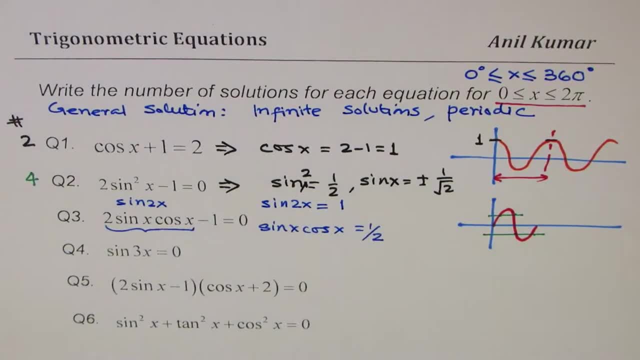 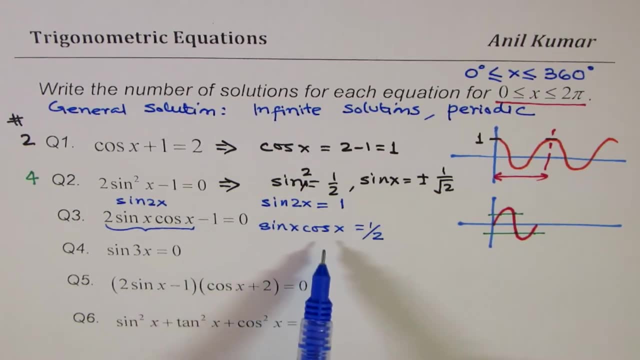 that is fine. as you can see, working with sine 2x equals to 1- you can also work with sine x. cos x equals to 1- is far better than working with sine x. cos x equals to half. so knowing double angle formulas is actually better. so we'll work with sine 2x equals to 1. now what is the meaning of? 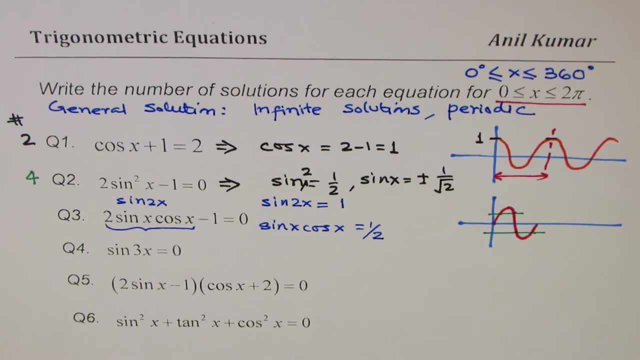 sine 2x equals to 1. now it really means that within the domain of 0 to 2 pi we have two sine waves, right? so let me sketch this here: it really means that within 0 to 2 pi, we have two sine waves. 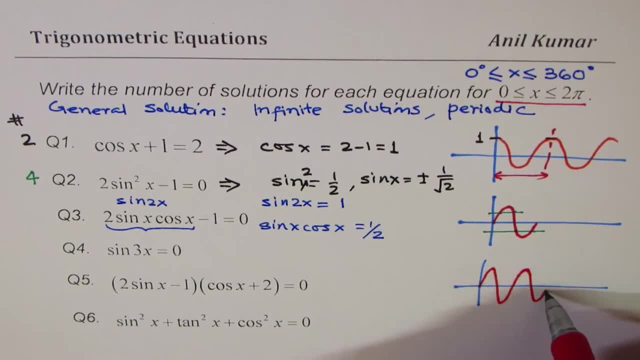 it's kind of like this: one and two. that is what it means. so this is for sine 2x from 0 to 2 pi. that was sine x from 0 to 2 pi. right, this was cos x from 0 to. this is 2 pi 4. so, as you can see from the graph, 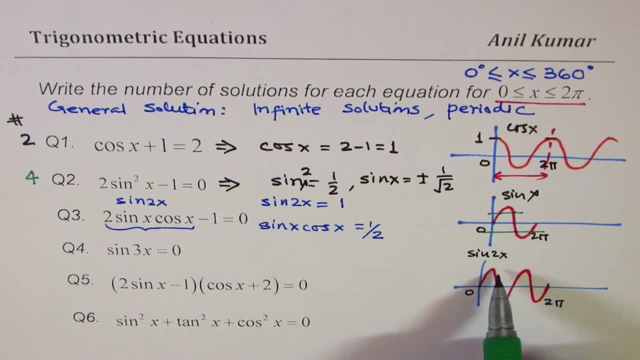 sine 2x equals to 1 means we have two solutions right, so we'll write two solutions for sine 2x equals to 1 or 2. sine x, cos x minus 1 equals to 0. does it make sense now, based on what you have learned so far? i would 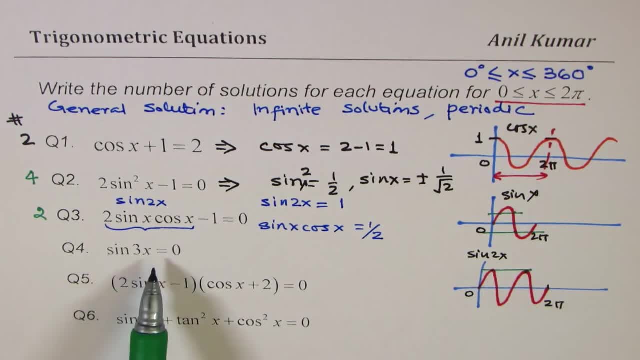 like you to answer this question. question number 4 sine 3x equals to 0. well, first step, let's try to sketch it. so if you sketch it within 0 to 2 pi, there should be three sine waves. so let's make three sine waves: 1, 2 and 3. so these are the three sine waves within 0 to 2 pi. we want that to be. 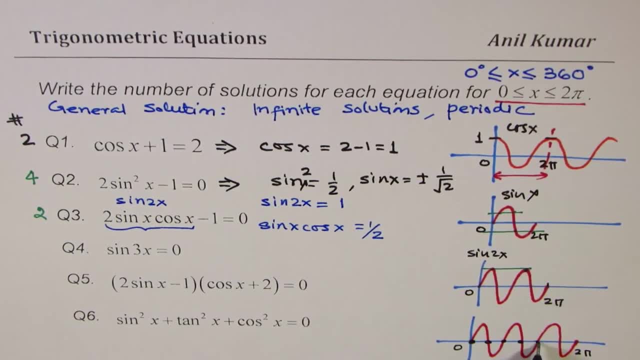 equal to 0. that means these are the zeros, the x intercepts, so you can count 1, 2, 3, 4, 5, 6, 7, so the answer is 7. do you see that? so sketching, visualizing and answering such question, really. 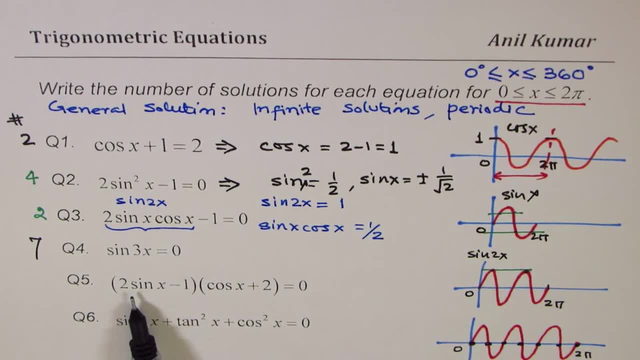 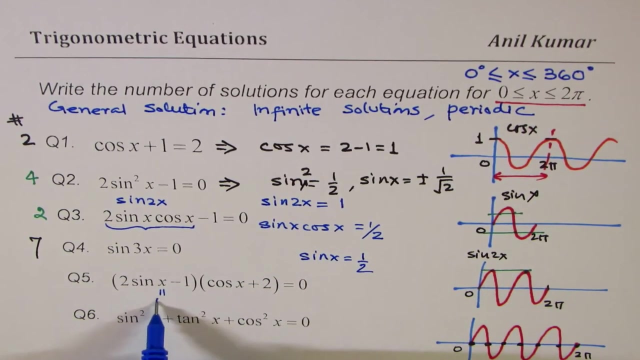 helps perfect. the next equation here is factored form of a quadratic equation: 2 sine x minus 1 times cos x plus 2. so in these equations we are looking for two conditions. one is: sine x 1 equals to half, since this could be equated to 0, and this can also be equated to 0, right? 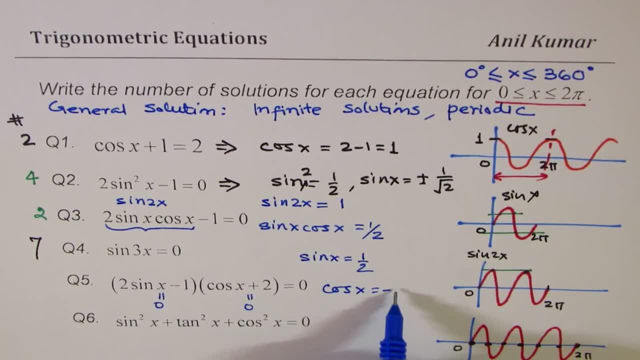 and we have cos x equals to minus 2. so these are the two possible solutions. correct: cos x equals to minus 2 does not give you any solution. so that no solution, since cos x value or sine x value is between plus minus 1. so we are. 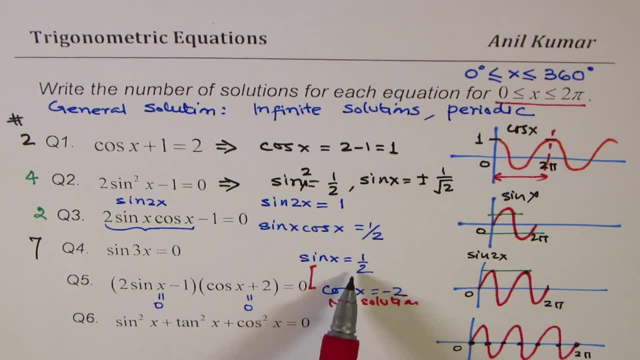 left with only one factor which could give us a real solution here. sine x equals to half means, a situation which we had just discussed earlier. right? so sine 1 wave in 2 pi, and there are two positions, so the answer for this will be 2. the last question here is sine square. 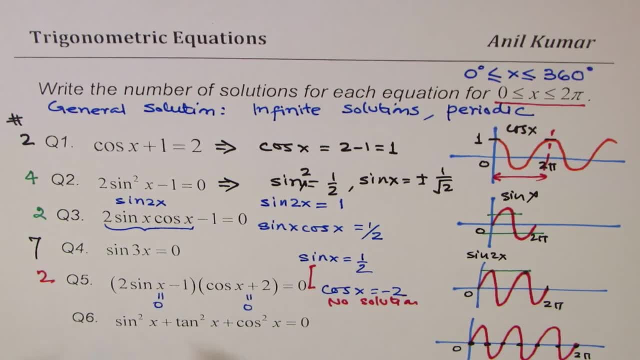 x plus tan square x plus cos square x equals to 1. you may have to work a little bit. sine square x plus cos square x is what right? let me rewrite: we have sine square x plus cos square x plus tan square x equals to 0. now this portion is 1, so we have 1 plus tan square x equals to 0, right. 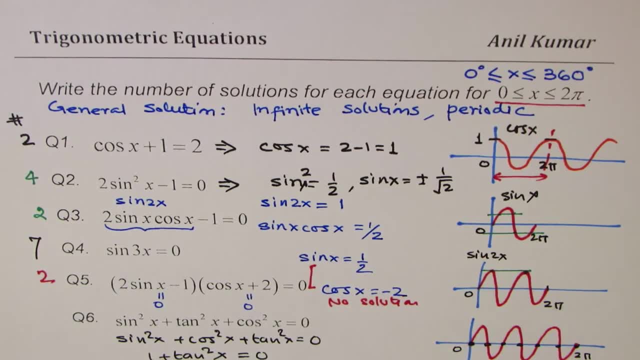 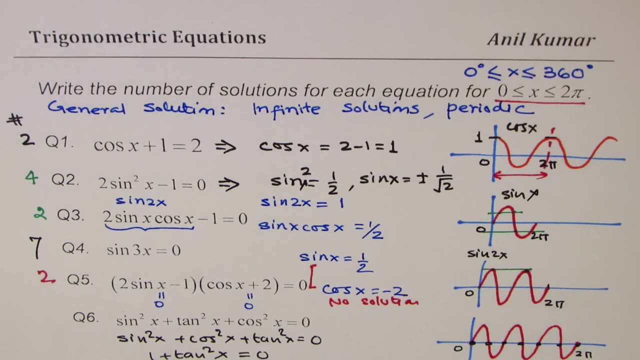 so that literally gives you tan x. equals to what? if i write minus, then you will say: well, there is no solution, correct. but what is 1 plus tan square x? well, you could say here: no solution, perfect, since 1 plus a square quantity, that means a. 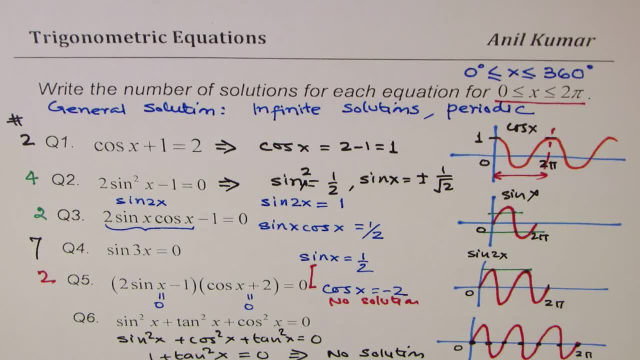 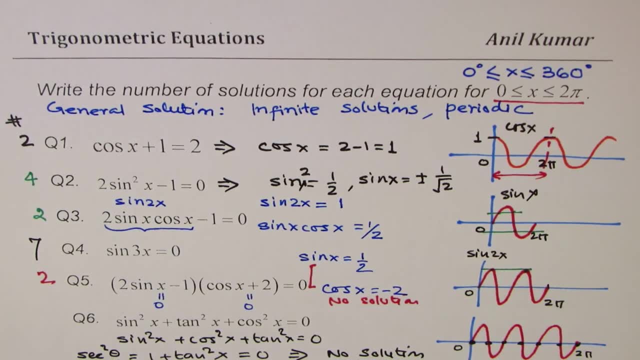 positive number cannot be 0, right? you can also try with secant square x. this is also equal to secant square x, but but you know, secant square x, the values are greater than 1 or less than minus 1, so that also will not give you any solution, right? so either way you follow, you will get no solutions.